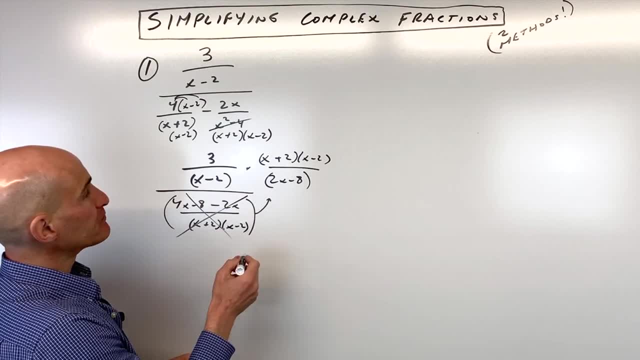 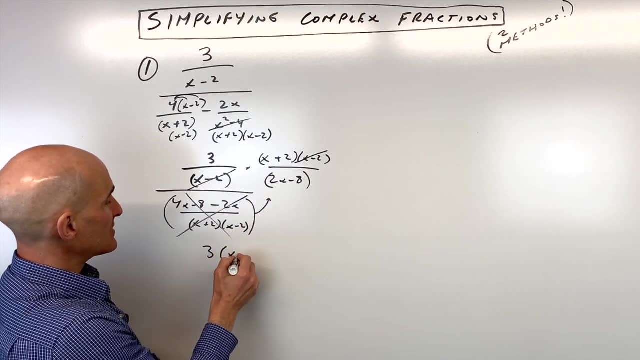 by the reciprocal. Now what we have is- let me just cross that out- you can see that the x minus twos are going to cancel numerator and denominator And we're just left with three times x plus two all over two. I'm going to factor this: 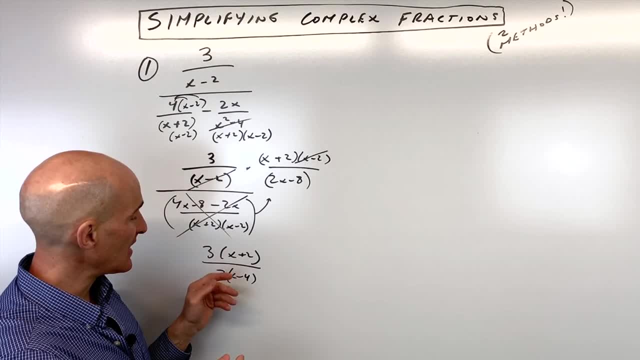 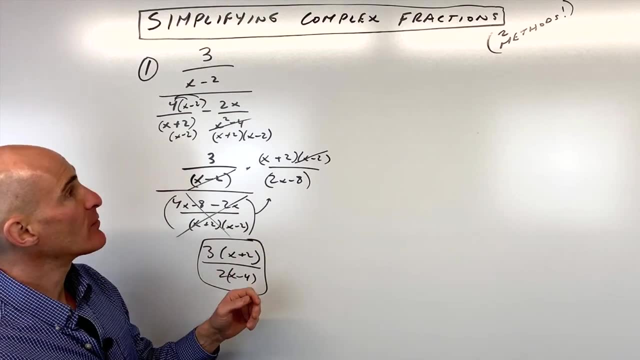 times x minus 4.. And the reason I factored is because sometimes you get some cancellation on numerator and denominator, So it's good to keep it factored and see if you can reduce. So this is our final result. Now let me show you method number two. So method number two. 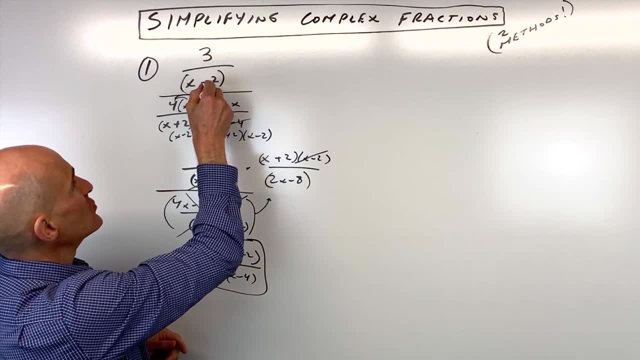 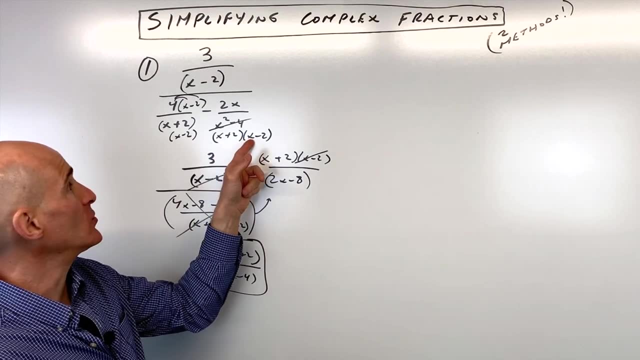 you would say: okay, let's look at all the denominators. We have an x minus 2.. Here we had an x plus 2, right, And here we had an x plus 2 and x minus 2.. So what we would do is we'd. 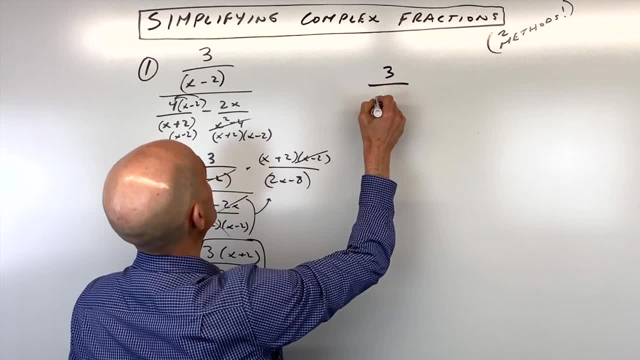 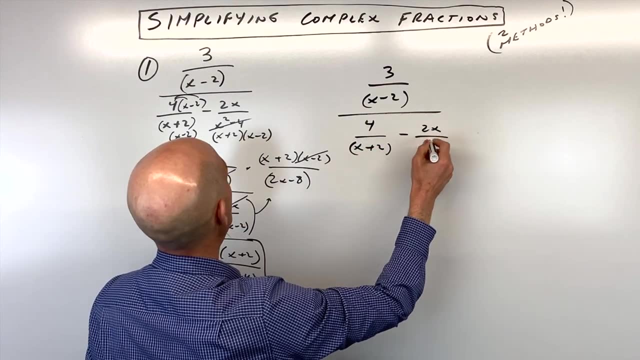 multiply through by the common denominator. Let me start by rewriting it so we can see a little bit clearer. So we have 3 over x minus 2, and we have 4 over x plus 2, and we have 2x over x plus. 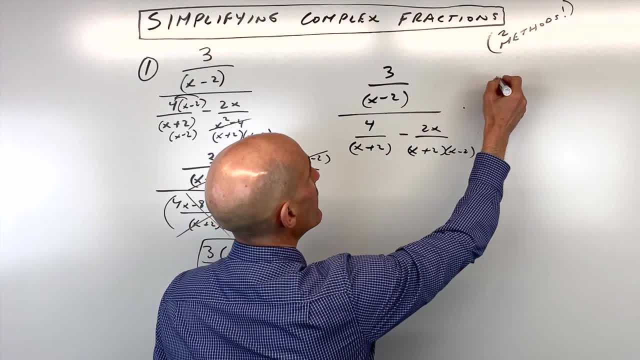 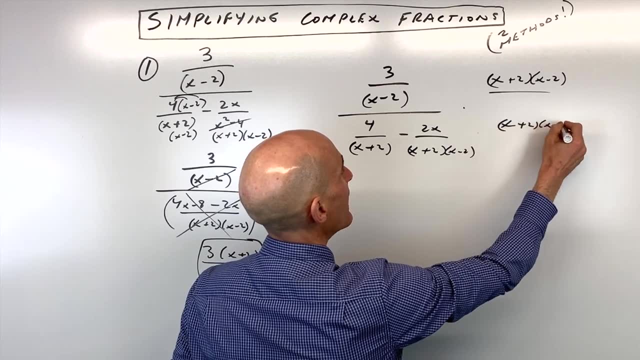 2, x minus 2.. But what we're going to do is we're going to multiply by x plus 2, x minus 2 to the numerator and the denominator. So anything divided by itself is 1.. So when you multiply by 1, it's. 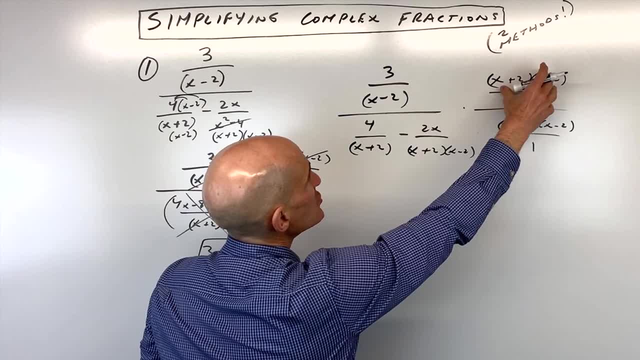 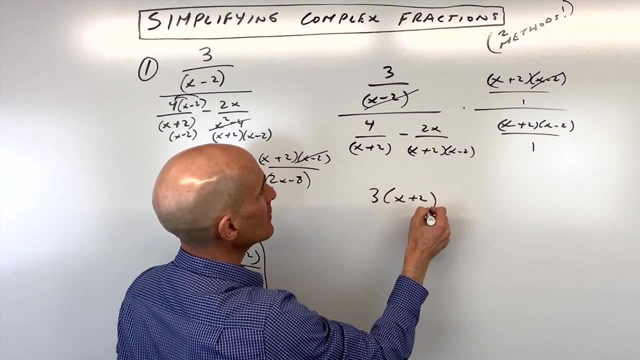 not going to change this fraction. It's just going to change the way that it looks. So when we distribute this here, it's going to change the way that it looks. So when we distribute this here, notice how the x minus 2s cancel. So we just have 3 times x plus 2.. In the denominator: 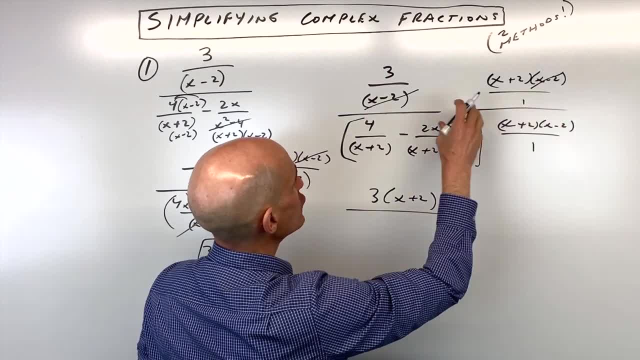 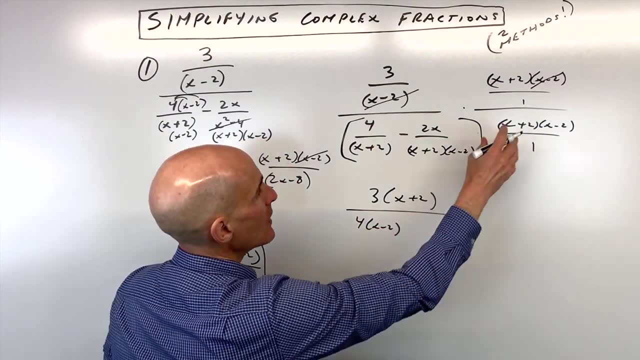 here. when we take this and we distribute it- this group- to the first fraction, you can see the x plus 2s are going to cancel. So you're just going to have 4 times x minus 2.. When you distribute this to the second fraction, what happens is that x plus 2, x minus 2 cancel and 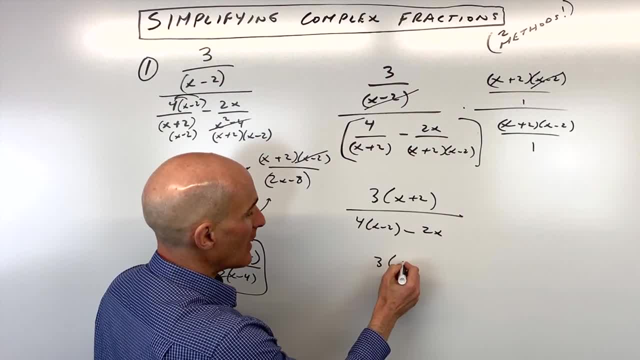 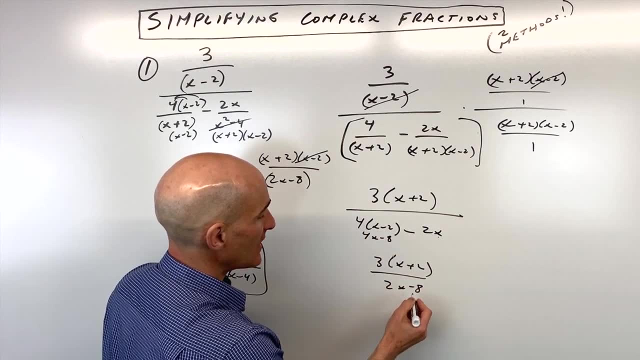 you're just left with 2x. So if we simplify this down a little bit, we have 3 times x plus 2.. So we have 4x minus 8 minus 2x, which just gives us 2x minus 8.. And then we can factor that. 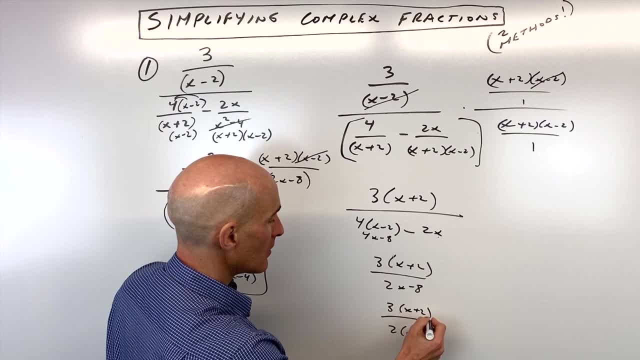 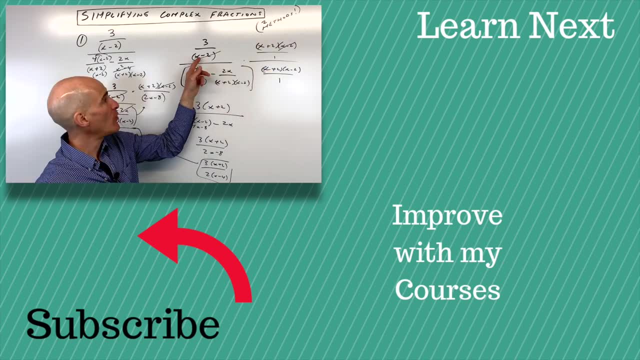 denominator again, like we did before, And you can see we're getting the exact same end result. So either clear the denominators by multiplying through by the common denominator or combine your fractions in the numerator to get one fraction and the denominators to get one fraction.